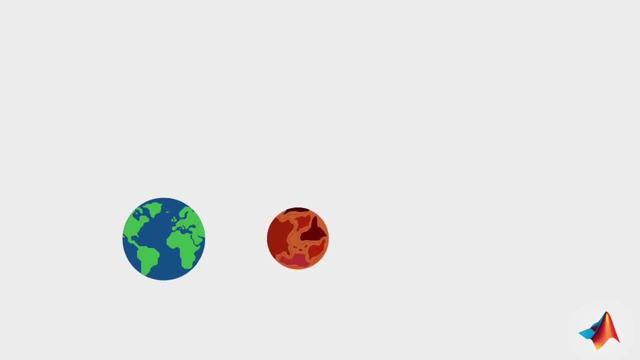 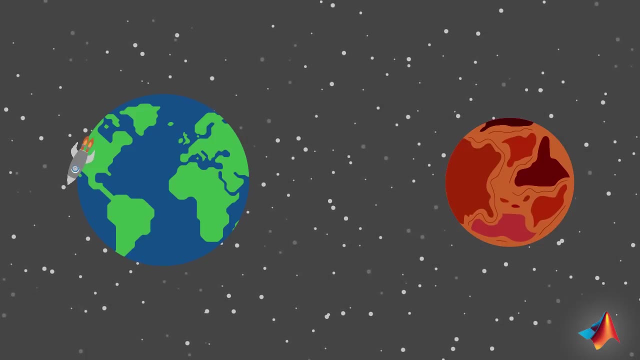 when it cannot be measured directly. To illustrate this, let's go to Mars before anyone else does. If your spacecraft's engine can burn fuel at a high enough temperature, it can create thrust that will let you fly to Mars. By the way, according to NASA, liquid hydrogen is a light and powerful rocket propellant. 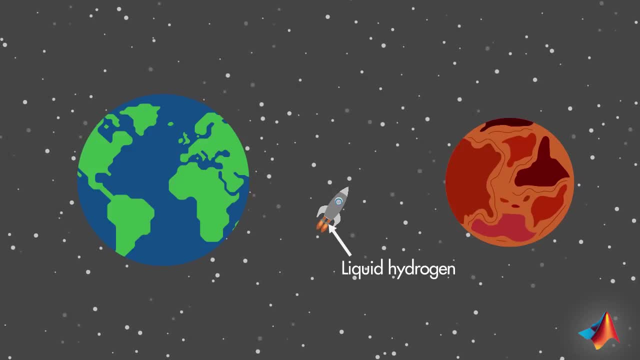 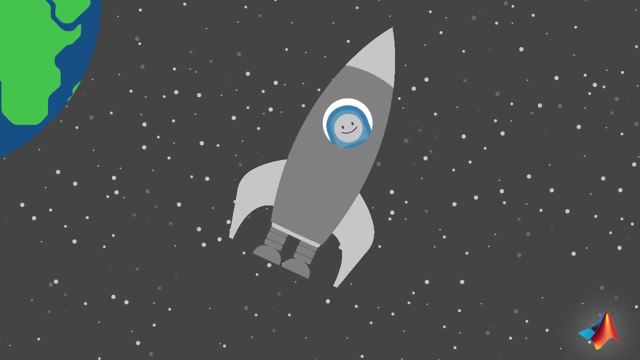 that burns with extreme intensity at 5500 degrees Fahrenheit. But be careful, because a too high temperature can put the mechanical components of the engine at risk And this can lead to the failure of some of the mechanical parts. If that happens, you might be stuck in your small spacecraft where you got to eat from. 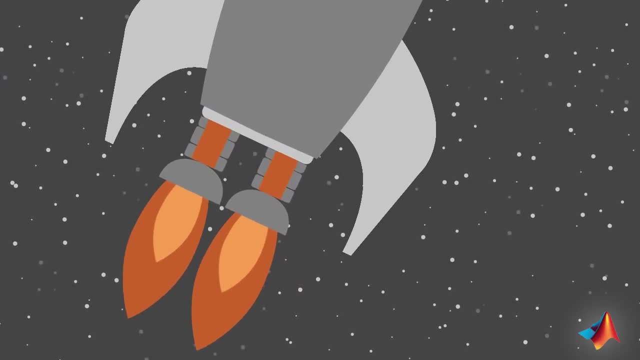 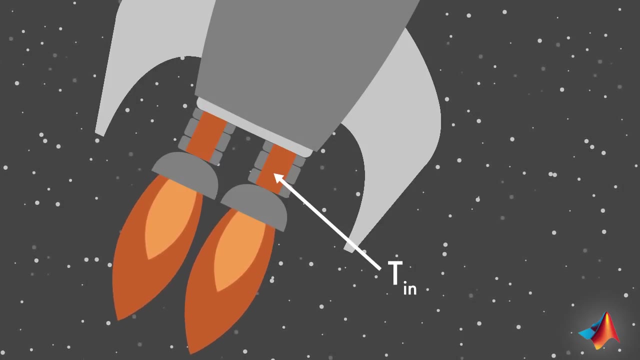 tubes. To prevent such a situation, you should closely monitor the internal temperature of your spacecraft. This is not an easy task, since a sensor placed inside the chamber would melt. Instead, it needs to be placed on a cooler surface close to the chamber. 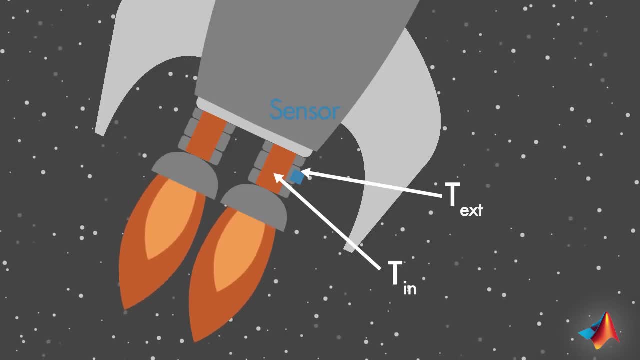 The problem you're facing here is that you want to measure internal temperature of the chamber, but you can't. Instead, you have to measure external temperature. In this situation, you can use a Kalman filter. You can use a Kalman filter to find the best estimate of the internal temperature from. 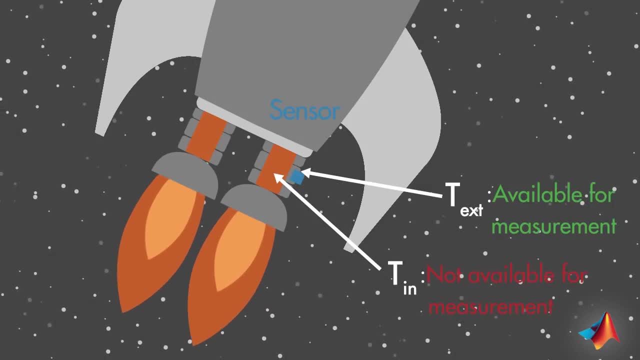 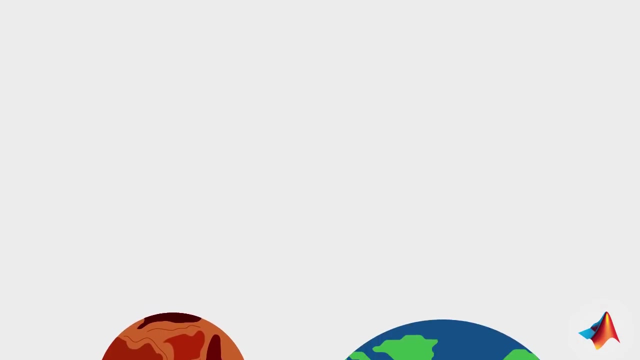 an indirect measurement. This way, you're extracting information about what you can't measure from what you can. Now that you know the solution to your problem, you can continue your journey to Mars. But are you scared of traveling in space? Let me tell you this. 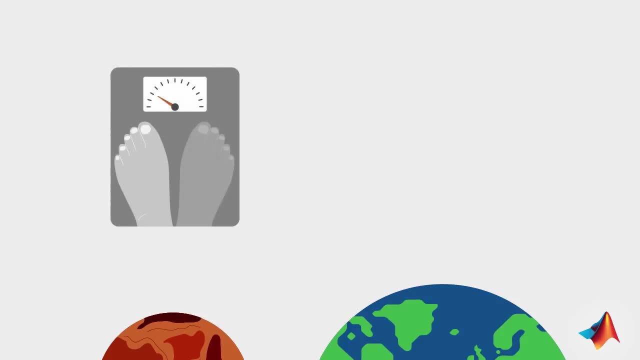 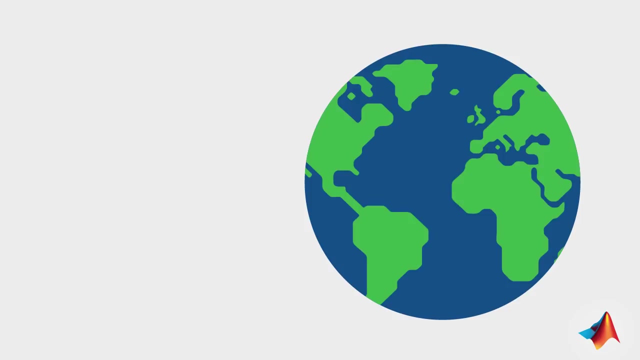 On Mars, you're going to weigh 60 tons, 62% less than what you weigh on Earth. Still not convinced? Okay, then let's go back and take a look at another scenario that takes place on Earth. In this example, we're going to see how a Kalman filter can be used to estimate the 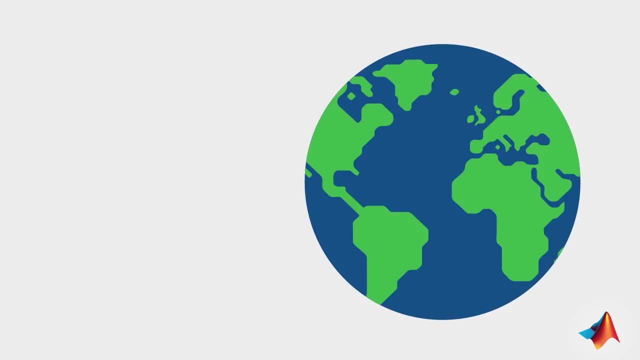 state of the system by combining measurements from different sources that may be subject to noise. You have guests visiting from overseas And you need to pick them up from the Earth And you need to pick them up from the airport. You're using your car's navigation system. 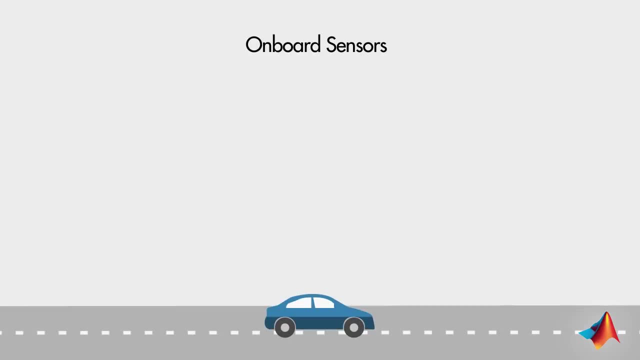 Let's look at the sensors you have on board, which help you find your position and navigate you to the airport. The inertial measurement unit uses accelerometers and gyroscopes to measure the car's acceleration and angular velocity. The odometer measures the relative distance traveled by the car. 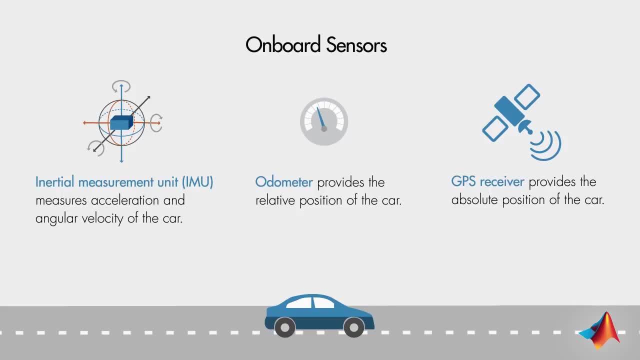 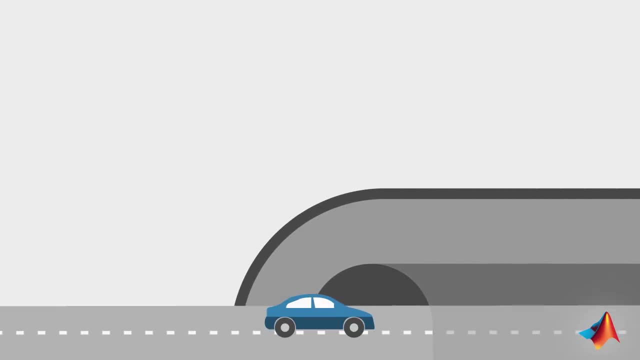 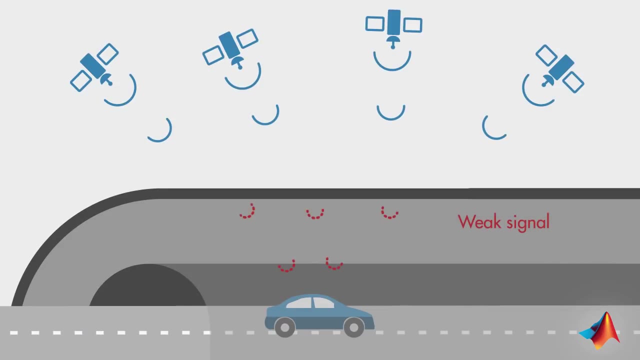 receives signals from satellites to locate the car on Earth's surface. If you live in Boston, as I do, you've got to travel through the Big Dig, a very, very long tunnel, And in the tunnel it gets harder to estimate your position through GPS, since the receiver's line of sight to 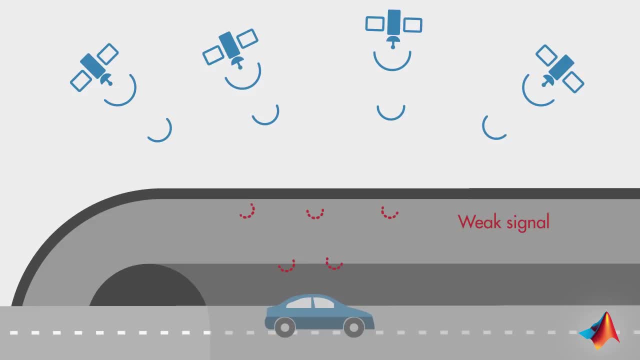 satellites is blocked and the GPS signal is weak. In this case, you may want to trust the IMU readings, which give you the acceleration. However, acceleration itself doesn't tell you much about the car's position. For that, you need to take the double integral of the acceleration. 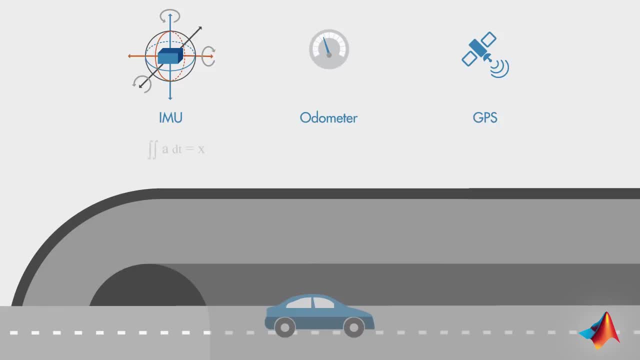 Unfortunately, this operation is prone to drift due to small errors accumulating over time. Thank you. To get better position estimates, you can use IMU measurements along with odometer readings, But note that odometer measurements may be affected by the tire pressure and road conditions. 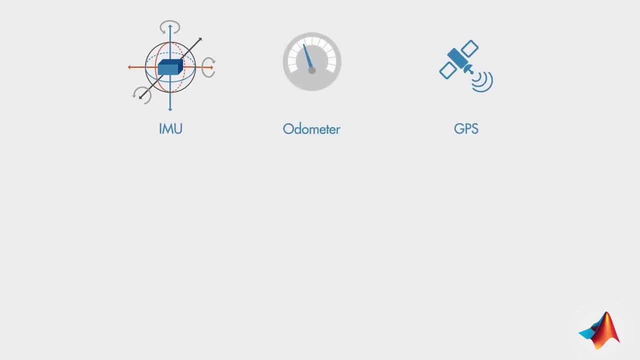 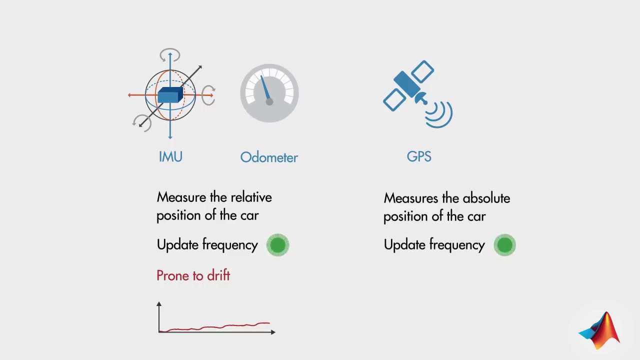 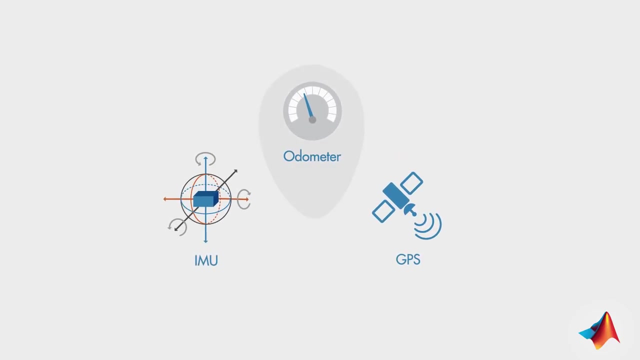 To summarize: your sensors measuring the relative position of your car give you fast updates, but they are prone to drift. The GPS receiver provides your absolute location, but it gets updated less frequently and it may be noisy. In this scenario, a Kalman filter can be used to fuse these three measurements to find the optimal estimate of the exact position of the car. 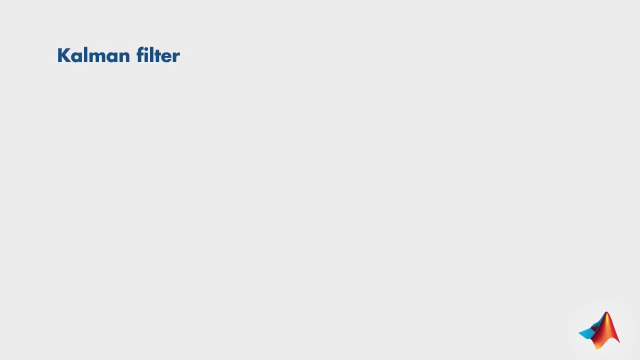 Let's look at some facts about Kalman filters. The Kalman filter is named after Rudolf Kalman, who is the primary developer of a sensor. It is an optimal estimation algorithm that predicts the parameters of interest, such as location, speed and direction, in the presence of noisy measurements.